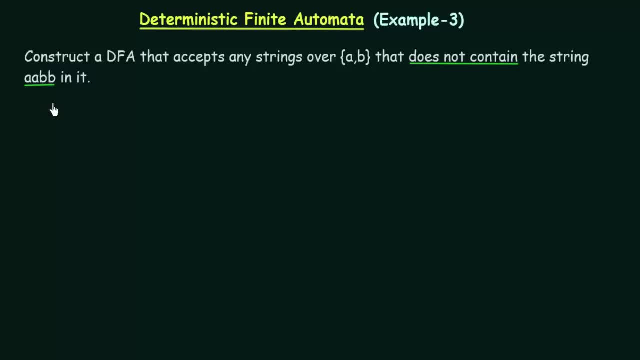 always accept all other sequence. So how can we do this? So here our alphabet sets or our inputs are A and B. OK, A and B are our alphabet sets or our inputs. Okay. so when we see this question we may think: how can we do this? This seems to be a very tough job. 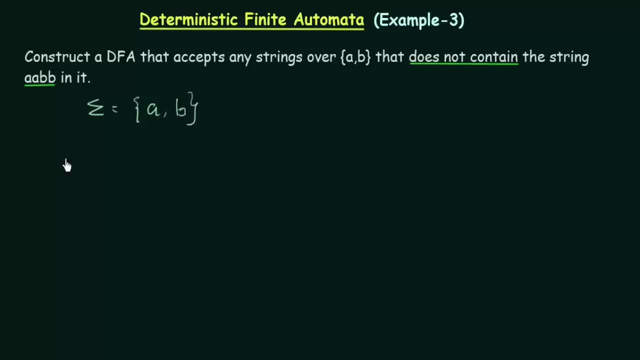 Okay, it's not very tough job. We can simplify this problem Instead of doing this right away. we can simplify this problem and make this problem simpler. So let us try to design a simpler problem. Let us modify this question in order to make it simple. Now, how can we do this? 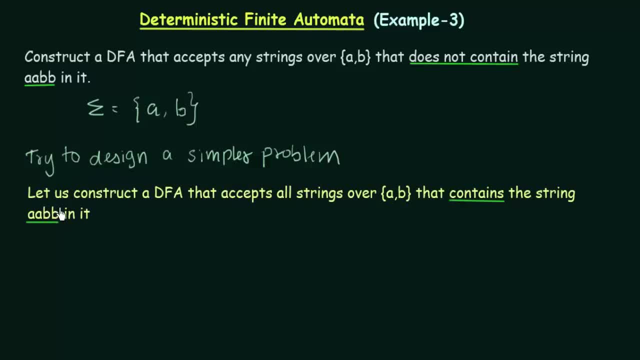 Okay, so here is how we simplify this problem. Instead of constructing a DFA that does not contain information, Let us construct a DFA that accepts all string over AB that contains the string AABB in it. I think that is more simple. We can construct a DFA over AB that contains the string AABB in it. 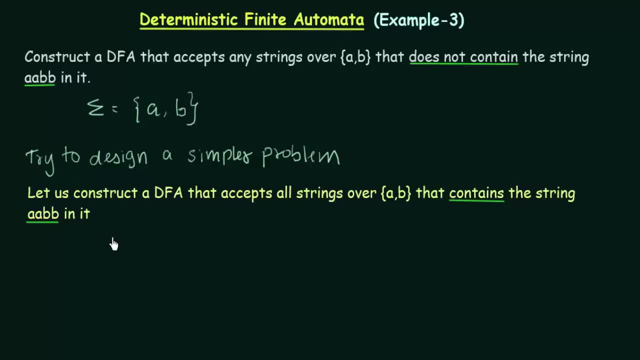 Alright, let us first construct this. This seems to be, this sounds to be more simple, So let us construct this, and later we will convert it to this form. Alright, so let us see how we can do this. So when you, whenever we start constructing a DFA, what we? how do we first start? 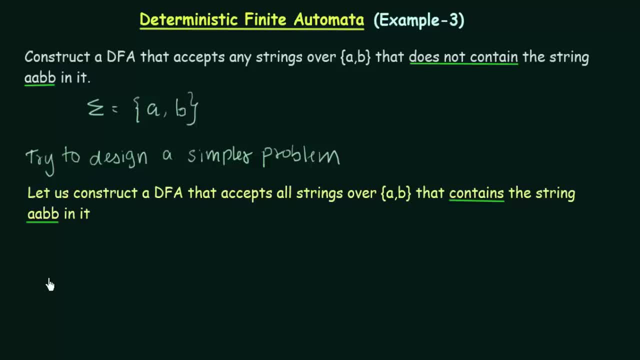 We need to have a starting state. So here I'll have my starting state as A, I'll call it A and I give an arrow this way indicating that this is a starting state, And A can either get inputs A or B, right. 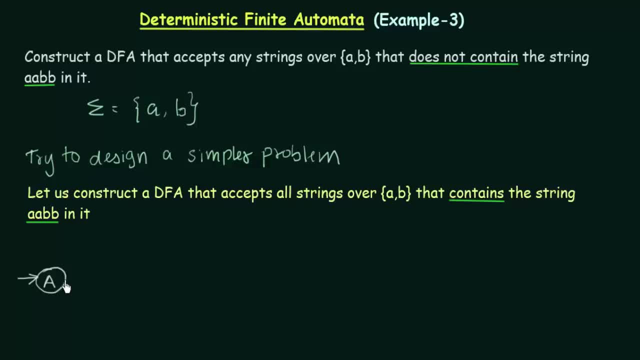 So what happens when it gets input A and what happens when it gets input B? So if A gets the input Small letter A, then what happens? I will send it to the next state, which I will call state B. Why? 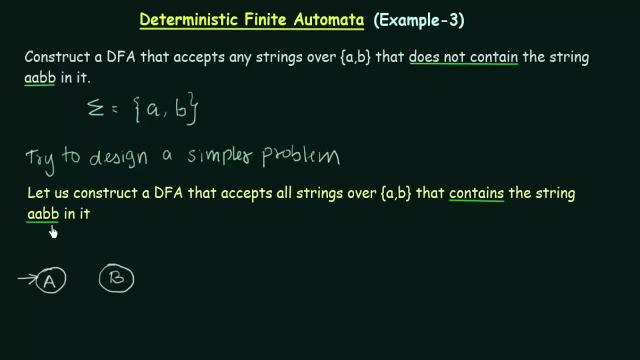 I need to get this sequence. AABB right. It should accept everything that contains this sequence. So when A gets the input small a, it goes to B. Yeah, I want it to proceed. Why? Because I am trying to get this sequence. 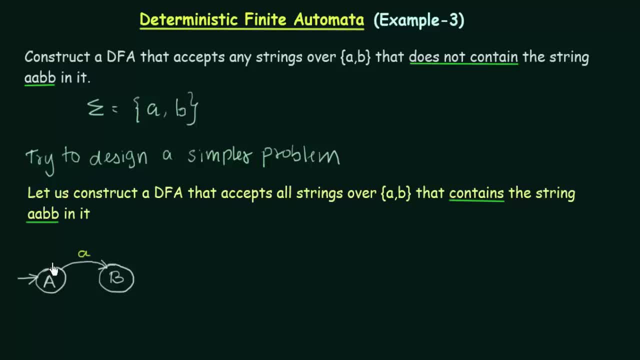 Okay, And what about when A does not get? when A gets the input small b, right, If A gets the input small b, I let it stay in A itself. If it gets B, it stays in A itself, because B should not be my starting letter. 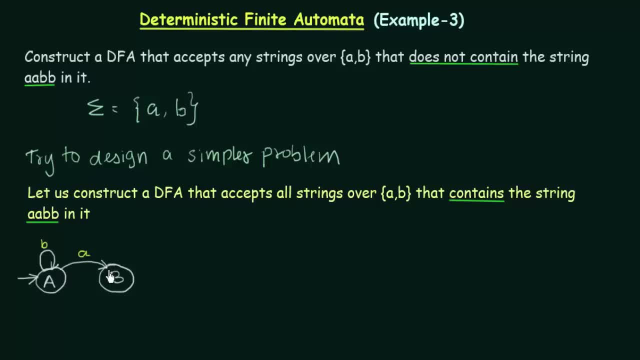 It should be A. So if it gets A it proceeds to the next state, But if it gets B, it stays in A itself. Okay, Now I got A and I came to state B. Now what happens in state B? 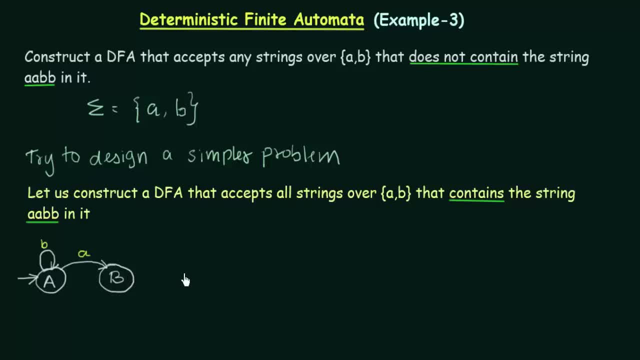 In state B. if I get the input A, what will happen? And if I get the input B, what will happen In state B? if I get input A, I send it to the next state, which I call state C. Now, why do I do that? 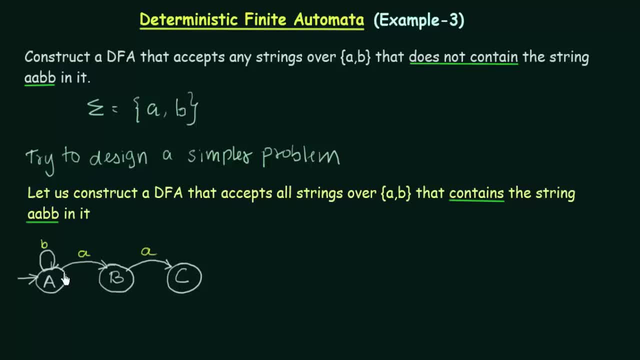 Because I want the sequence AABB. Okay, So I get the first A and I got the second A. Right, This is the second A, So I proceed to the next state. But what if? what? if B gets the input small b, then it should go back to state A. 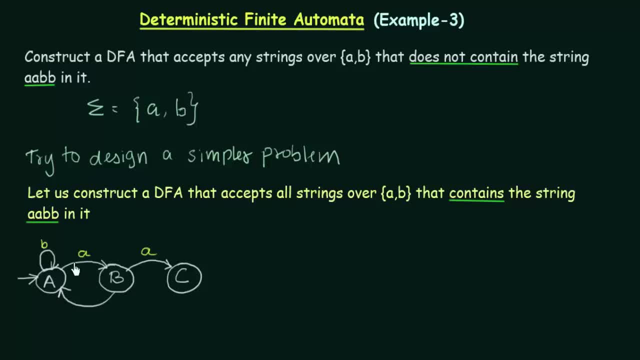 Why? Because if I get, after getting A over here, if I get another B, what happens? I got A, and if I get a B, then what happens? My sequence becomes AB. No, I don't want AB, I want AA. 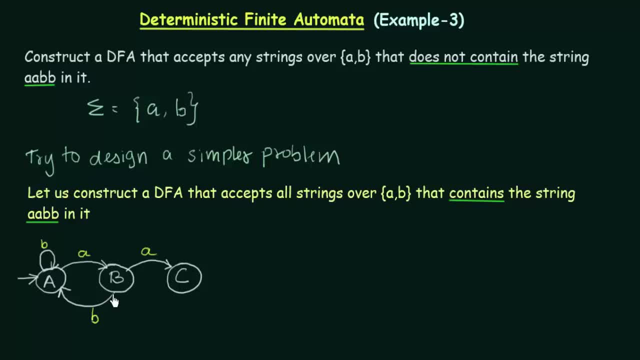 AA is what I want, not AB. So if I get B, I send it back to state A, So it will start again from here. So my state B is complete. I have already mentioned what happens if it gets A. 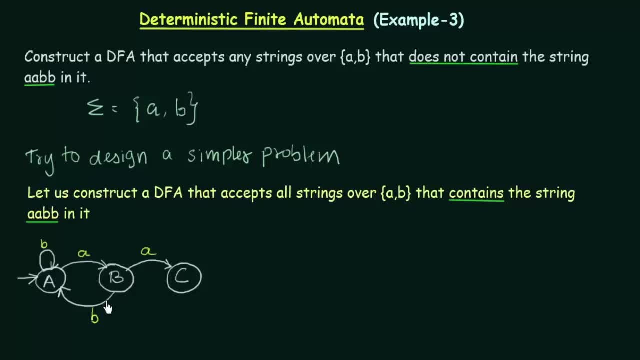 If it gets A, it goes to state C. If it gets B, it goes to state A. Okay, Now coming to state C. In state C, how should I proceed? I got AA. Now, if I get B in state C, I should proceed to the next state. 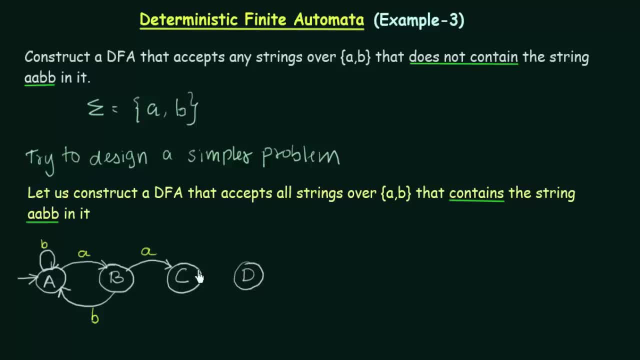 So I will call my next state as state D, and what is the sequence that I want AABB. So I already got AA over here. Now the next one is B. So if I get B, If I get B in state C, I let it proceed to the next state. 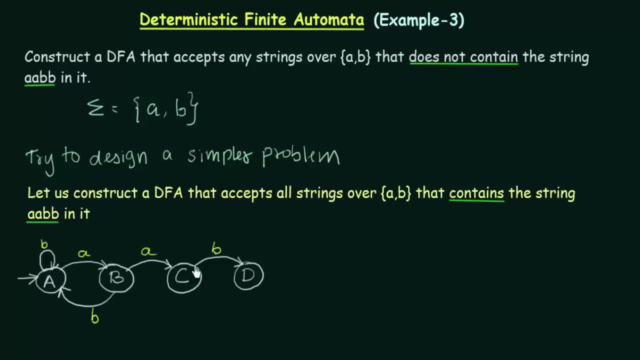 Okay, I let it proceed to the next state. And what if I get input A in state C? What will happen, or what should I do? So, in state C, if I get input A, where should I send it? Should I send it back to B, or should I send it back to A, or should I keep it in C itself? 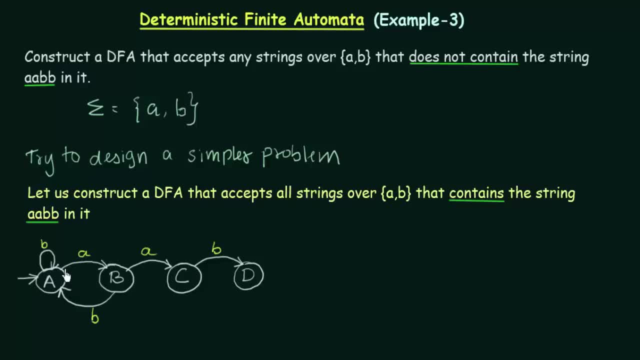 What I should do is I should analyze it this way: How did I come to state C? I came to state C from A to B and then from B to C, So we know that on reaching state C, we already got these two inputs. 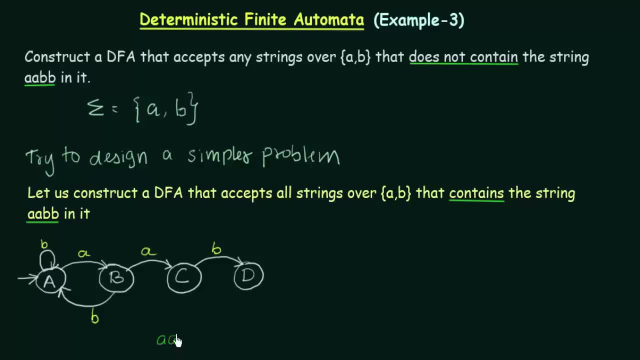 A and A. I already got AA And if I get B I go to state D. But what if I get A again? If I get A again, I don't need to send it back to state D. I can send it back to state B or state A. 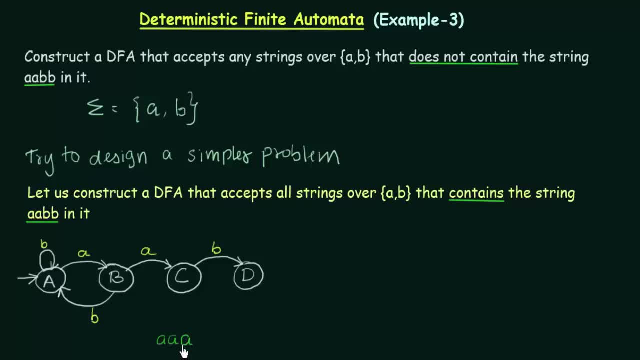 Why? That is because I already got 1,, 2,, 3.. And I could get B as my next Right. In the next one, I could get B. So that is why what I should do is I should keep it in state C itself. 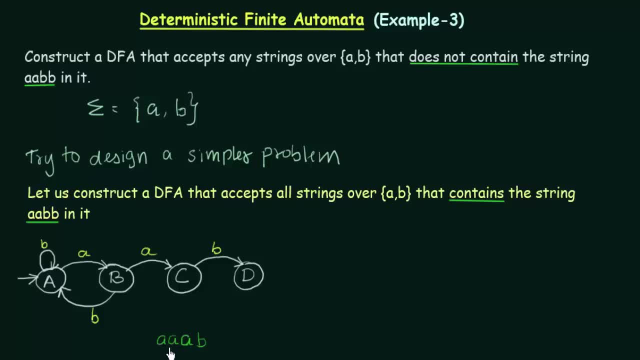 Right, Because if I am in state C itself, then I can count from here A, A, B, And if I get another B it will be accepted. I hope you are getting my point. So I keep this C in C itself, if the input is A. 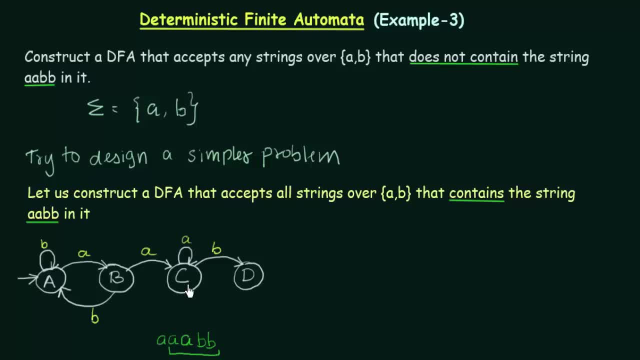 Right. So on reaching state C, if I get input B, I proceed, Because, yes, I can proceed. But if I get input A, that means it could mean something like this: Right, I get another A. So I keep it in this C itself. 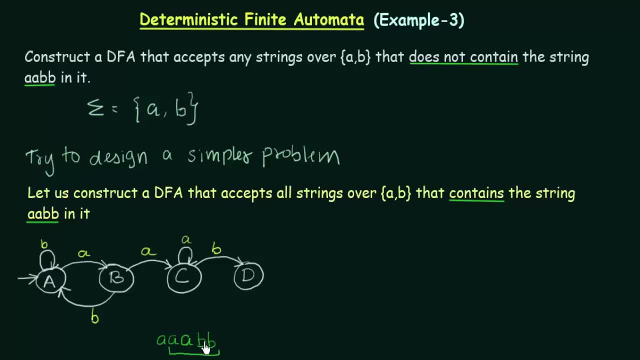 Because in the next input I may get a, B, So I keep it in C itself. So I hope that was clear. So my C is complete. I already mentioned what happens if I get A or B. Now coming to D: 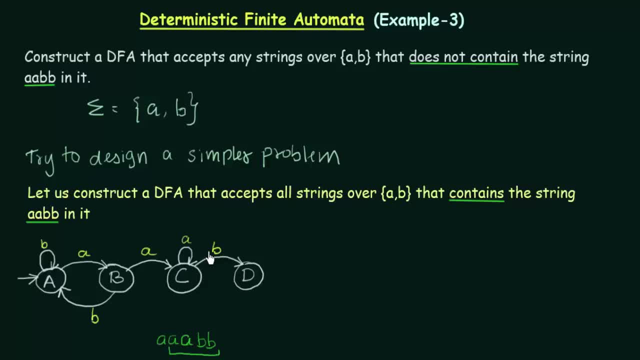 So, on coming to D, if I get input A, what will happen? If I get input B, what will happen? So, on reaching D, how many inputs did I get? I got A A, B. So I am here: A A, B. 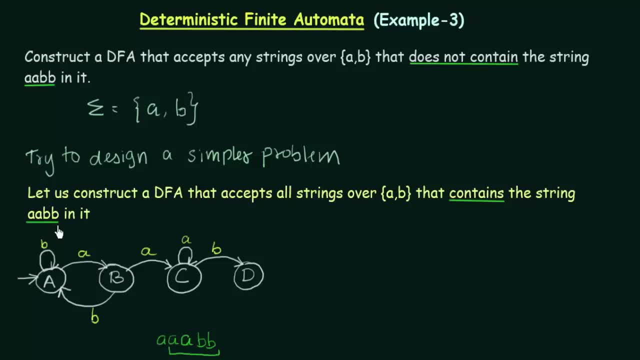 Now on state D. if I get the input B again, then I can proceed to the next state, which is state E. Right, And if I get B in state D, what is the condition of my input? It is A, A, B, B. 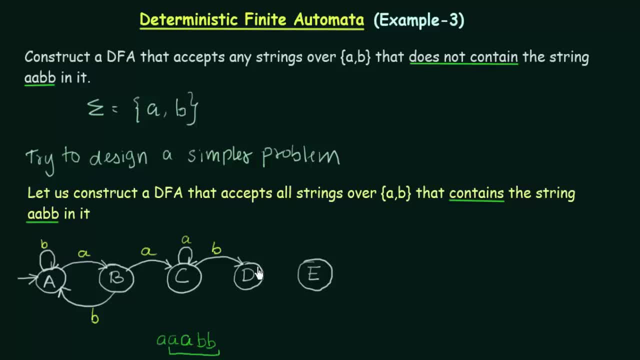 So this string is complete. So if I get B, it goes to state E and state E should be my final state or accepting state. State E should be my final state or accepting state coming from D. So I get A, A, B, B. 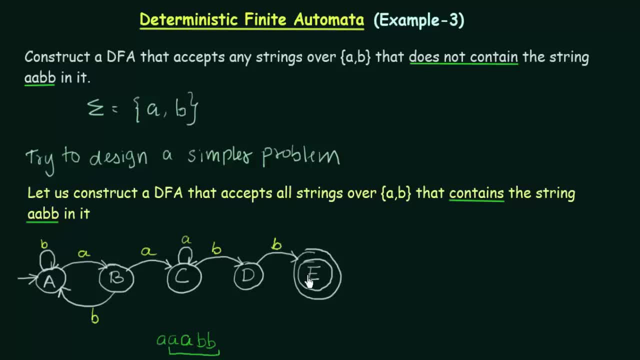 A, A, B, B, And when I reach here, this should be the final state, Right? So that is About state D, if I get input B. Okay, Now what will happen if I get input A in state D? 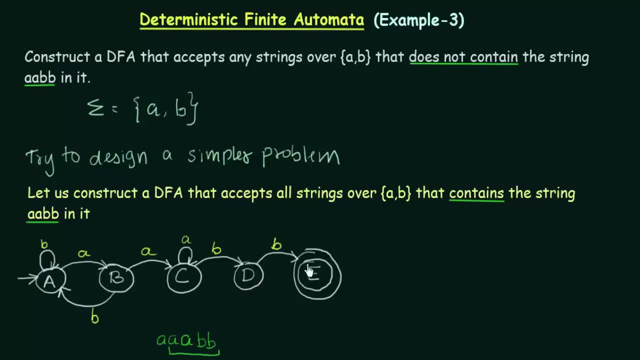 We already mentioned, if it gets input B, it goes to the final state. But if I get input A in state D, where should I send it back? Should I keep it in itself? Should I send it to C, B or A? 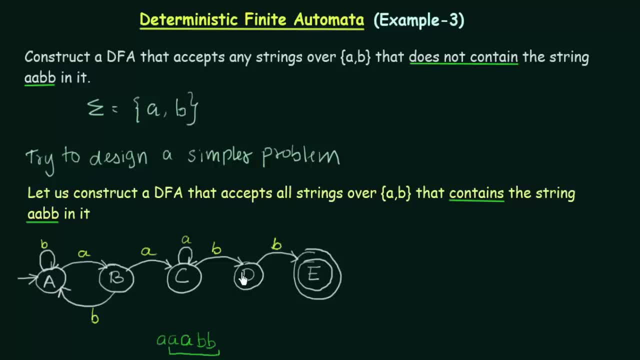 Let us check it out. How did we reach state D? What is the condition or state of our input when we reach state D? We came from A and we got another A and we got B, So we got A, A, B. 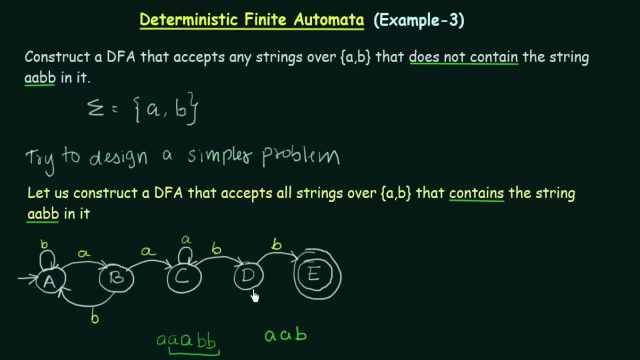 This is our condition: A A, B. Now our question is: if we get A again in this state D, what will happen? If I get A again over here, what will happen? I get this sequence: A A, B, A. 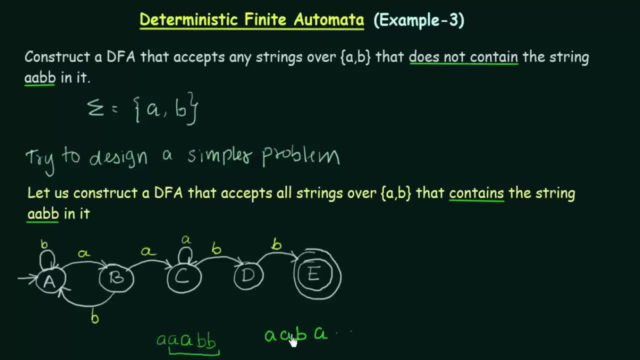 Now, even if I get A here or B here, whatever I get here, I am not able to get this sequence anymore. Right, I cannot get back this sequence whatever proceeds from here, So I have to send it back to this position where I got my first A. 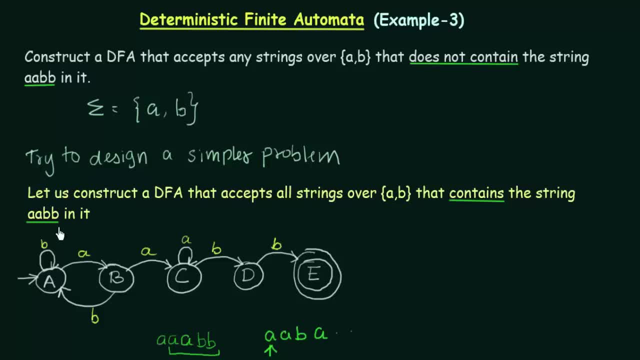 And then I have to try and see if it can get this A, A, B, B again. Right, I have to send it back to the position where I got my first A And where did I get my first A, My first A, I got over here. 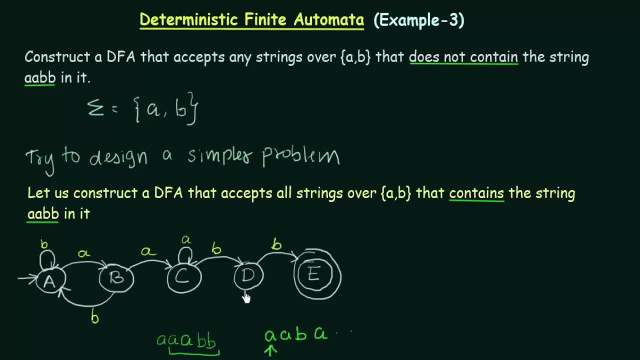 So, on getting first A, it reached state B, So I have to send this D back to state B. I have to send my D back to state B if I get the input A Right. So now my state D is complete. 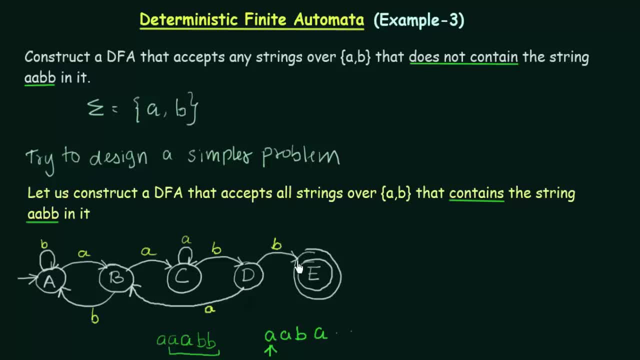 On getting A, it goes back here. On getting B, it reaches final state E. Now what is left? Our final state is left. We did not mention what happens if we get A or B in our final state. So in our final state. 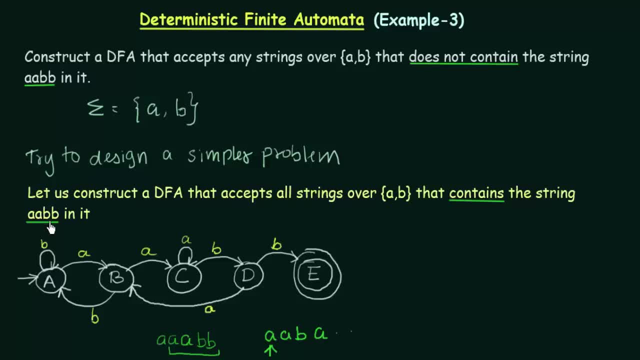 Okay, so when we reach our final state, we already got the sequence A, A, B, B. Now it does not matter what we get after that. Either we get A or B, it does not matter, It stays in the final state. 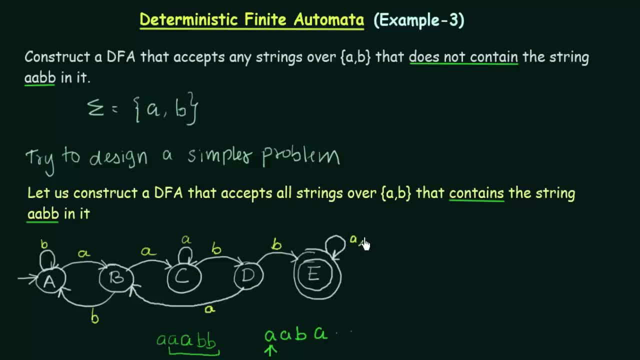 Right, It stays in the final state. A or B stays in the final state, So that completes our DFA, which accepts all string over A- B that contains the string A, A, B, B in it. Alright, Okay, so is that the end of our problem? 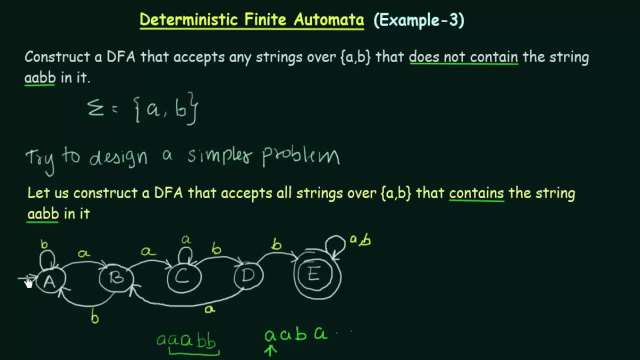 No, that is not the end of our problem, because we have now constructed the simplified problem. We have constructed a DFA that accepts all string over A, B that contains the string A, A, B, B in it. But our main problem was to construct a DFA that accepts all string over A, B that does not contain the string A, A, B, B in it. 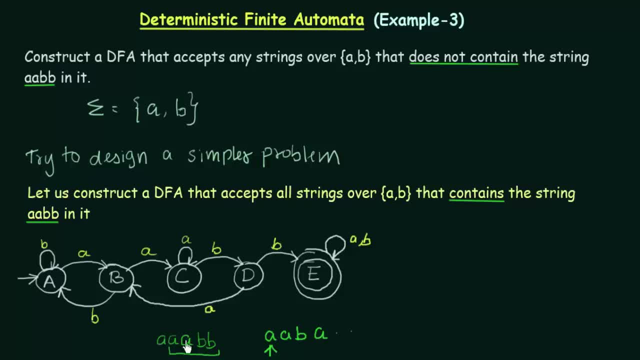 Now, how shall we do this? Now we have this. We have this DFA over here which accepts all string that contains A A, B, B. Now we need to flip this and make it in such a way that it does not accept A A, B, B in this. 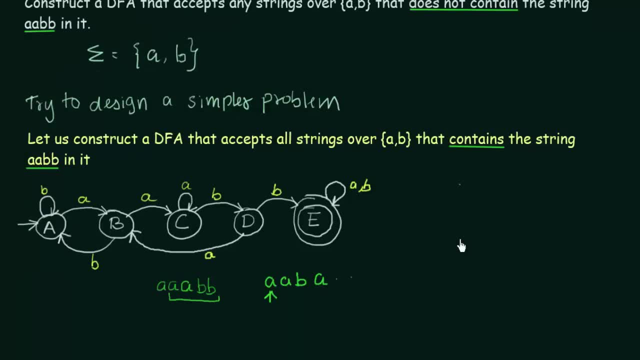 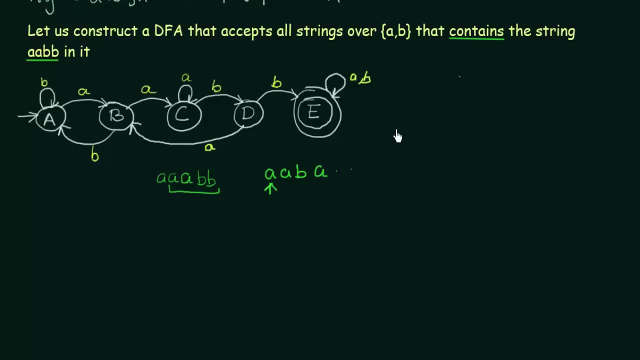 Now, how can we do this? How can we do this? This can be done in a very simple way, that is, by flipping the states. We can achieve this by flipping the states. What are we going to do? We are going to flip the states. 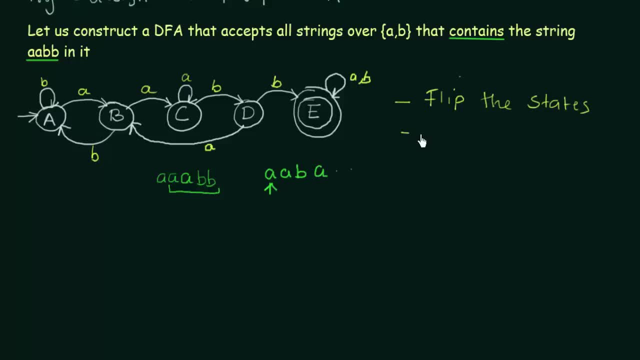 Now, what do I mean by this? What I mean by this is make the final state into non-final state and make the non-final states into final states. This is what I mean: to flip the states. To flip the states means to make the final states into non-final states. 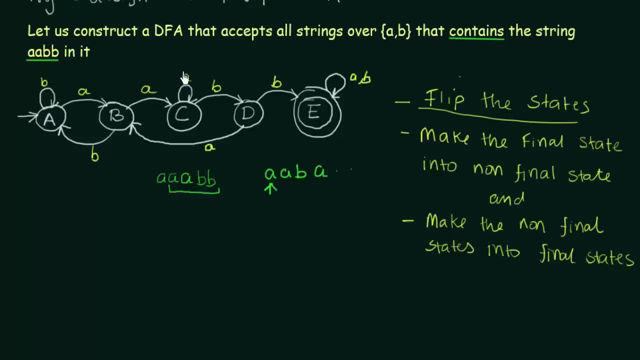 and make the non-final states into final states. In that way, we can make this DFA to accept all strings over A- B that does not contain the string A, A, B, B in it. Alright, Now let's see how we can do this. 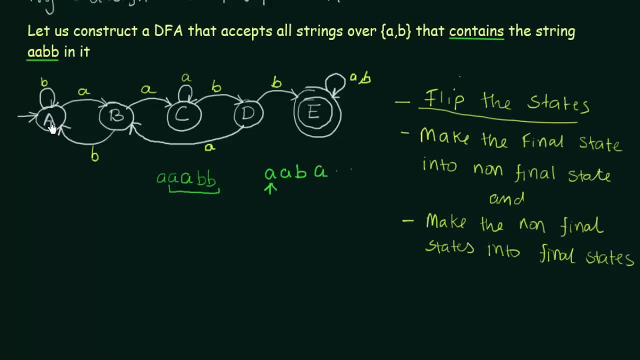 This is very simple: All these states here which are not final states, like A, B, C and D, make them final states, And the last state, E, which is a final state, make it a non-final state, And all the other things remains the same. 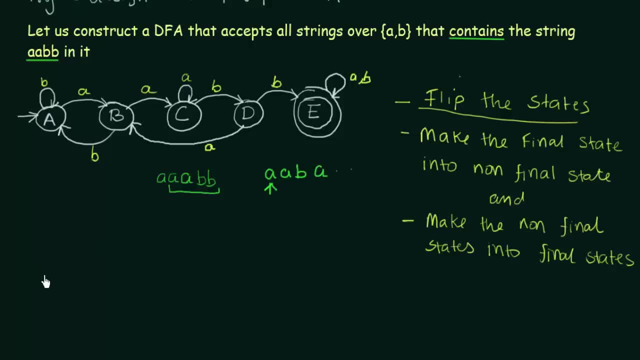 And then we can achieve a DFA, which was mentioned. So let us draw this. A was a non-final state, so I make it a final state. How? By putting a double circle around it. And this is the starting state. And B was also not a final state, so I make it a final state. 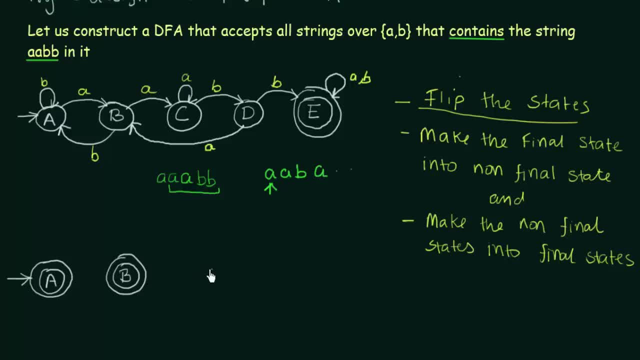 I put a double circle around it And C was also a non-final state. I make it a final state by putting a double circle And C, then D, which is also a non-final state. I make it a final state. I put a double circle. 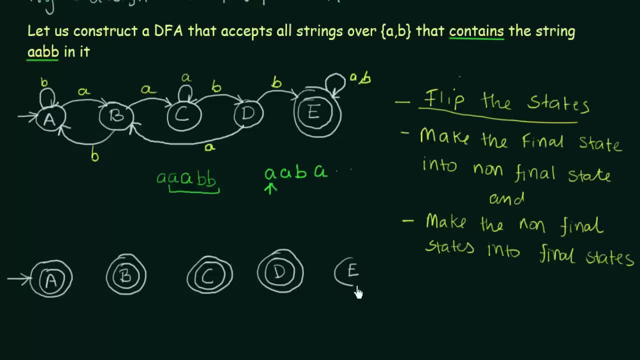 And E was a final state, I will make it a non-final state. I will give it only one circle. So all the rest of the things it remains the same. Just copy it down just as it was. It is all the same. 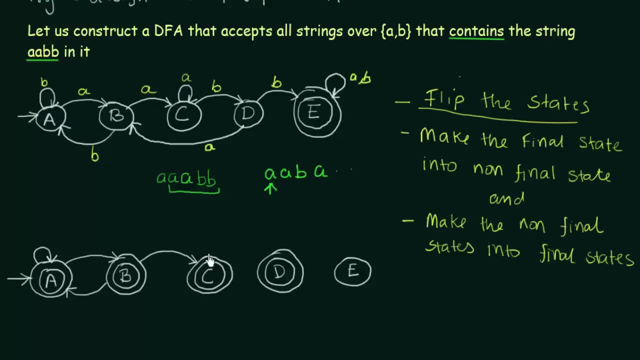 So this is how we can do it. Okay, C stays here And C goes here, And D goes to B And here, D goes to E And E stays in itself. And let us mention the inputs. Everything is same. 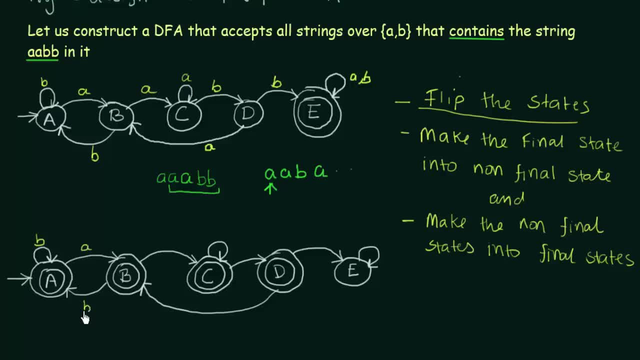 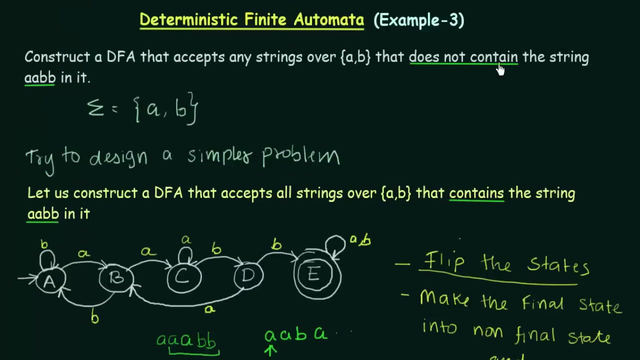 Just copy it down: B here, A, here, B here, A here, A, here, B, here, Another A over here And B here And here it is A and B. So this will now accept any strings over A, B that does not contain the string A, A, B, B in it. 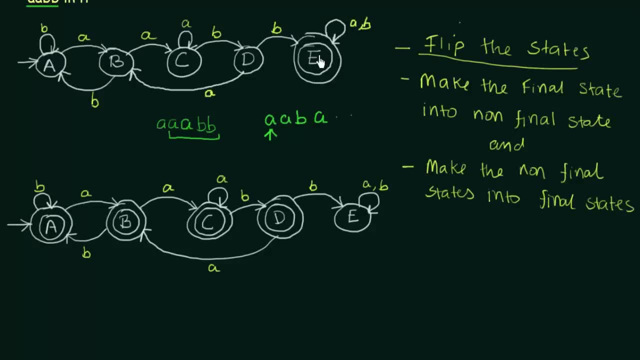 So we knew that when it reaches this E, it contains A, A, B, B Right, And it was accepted for this case. But in this one, whenever it contains A A, B, B, it reaches state E, which is not a final state, So that string will not be accepted. 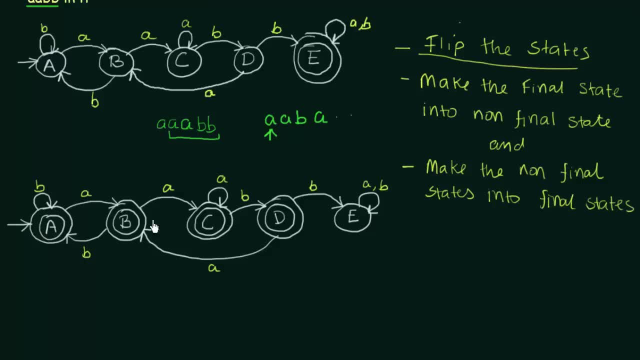 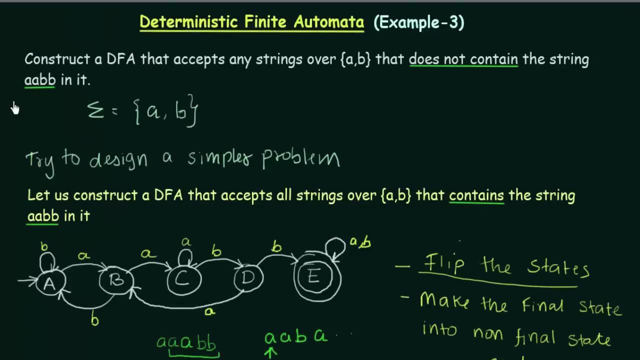 And all other strings will always be accepted in this for accepting states. So this is how we design a DFA for this kind of a problem. So whenever you get this kind of a problem, try to make it simple And then try to flip it. 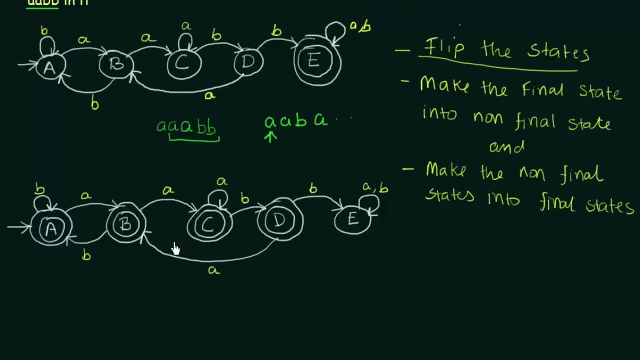 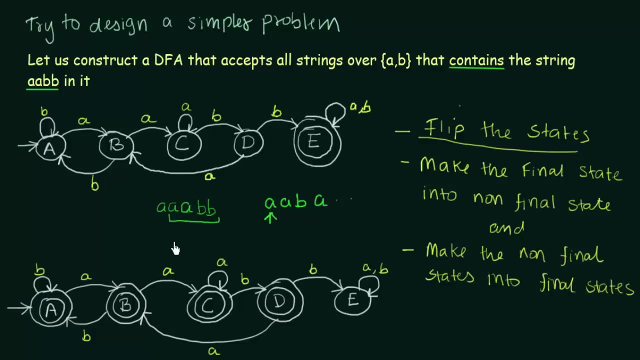 And make it work for the main problem. So I hope this was clear And please try to practice more of these kind of examples to make the DFA clear to you. So I hope this lecture was useful to you. Thank you for watching and see you in the next one.